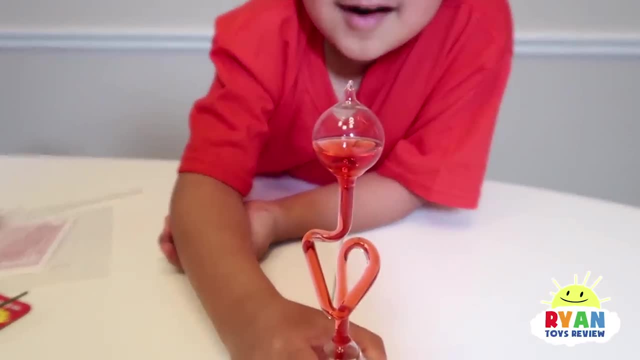 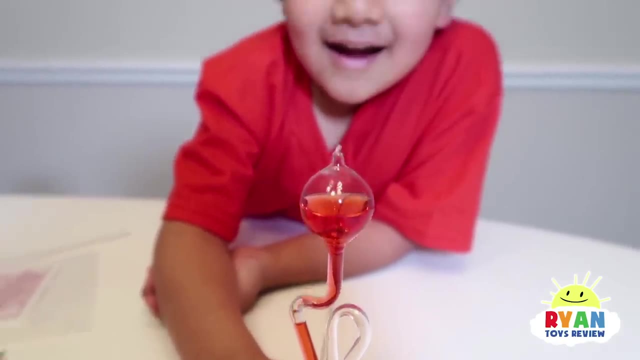 Oh, whoa, You see what's happening. It's filling up, It's going to the top. Let's see if it's going to reach the top. Ryan, you're boiling hot, Do you see? I guess Ryan is hot. Wow, look, it's going up, All right. 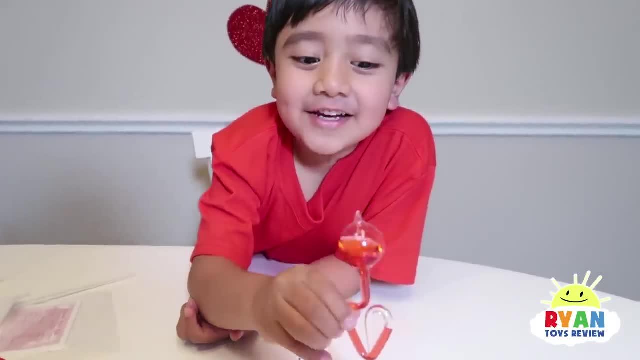 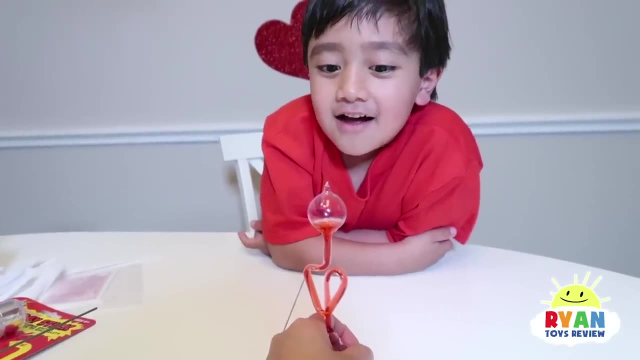 I'm going to test Mommy. Mommy, you're going to see if she's hot. Do you think she's hot? She's definitely hot. Let's see if Mommy is hot. I'm going to hold the bottom. Am I hot? 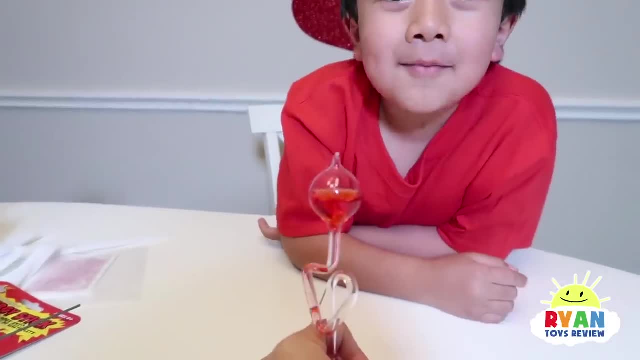 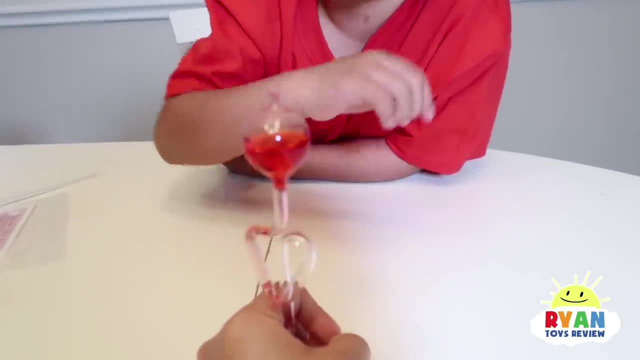 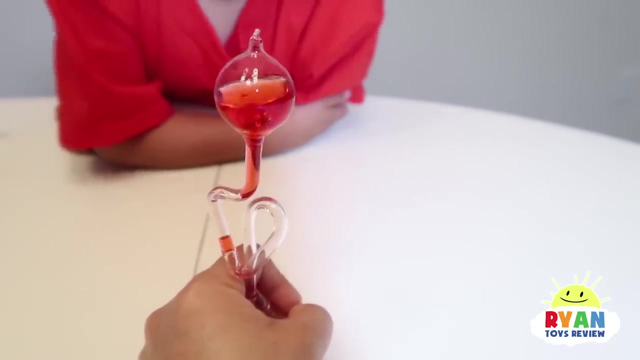 Is it going? Is it going? Come on, I guess Mommy is also hot. Look, it's going up. Do you see Mommy's more hot than me, because her hot went more faster. How does it work? The substance inside will boil at or below. 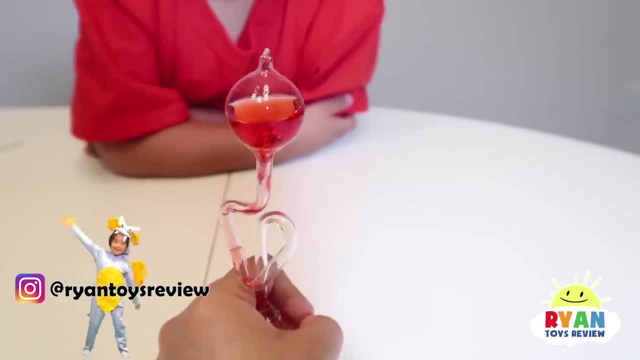 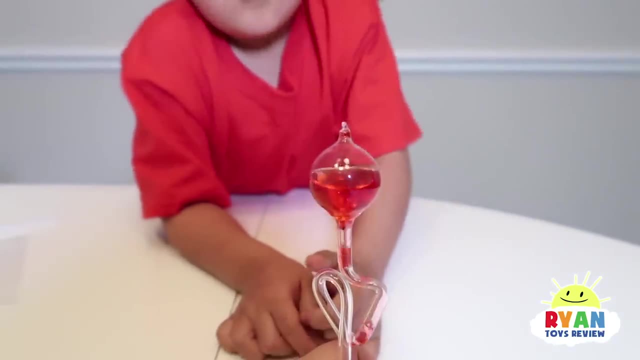 your body temperature 98.6 degrees, So that's why it boils. It's not really boiling when the heated gas push all the liquid out of the bottom chamber, Air bubbles are forced into the tube, So that's why it looks like it's boiling but it's not. But that's pretty. 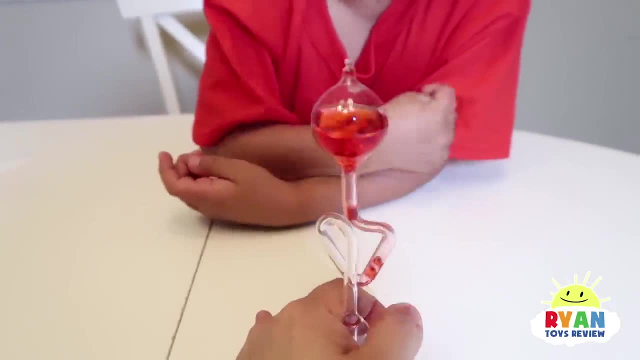 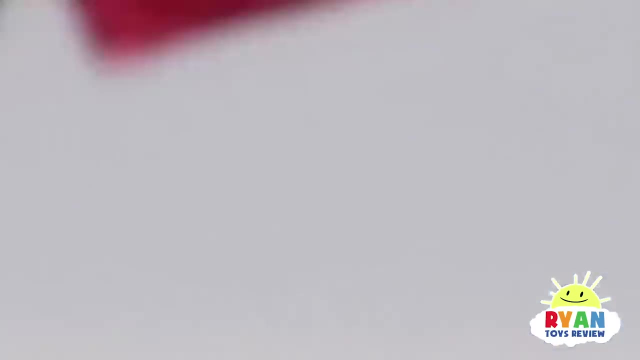 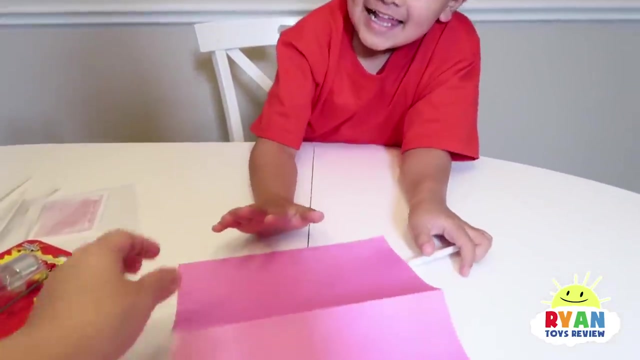 cool. It looks like all this stuff is twitching. Yeah. So experiment number one: Mommy and Ryan are both hot, Ding ding ding. Experiment number two: the ooh la la paper. Ooh la la. Okay, Ryan, so I need you to put your hand and put it down like a hand print. Let's see. 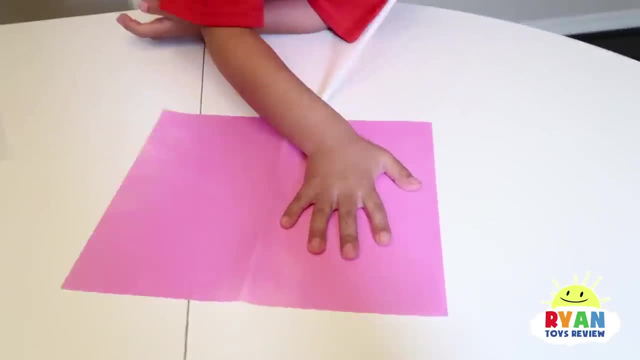 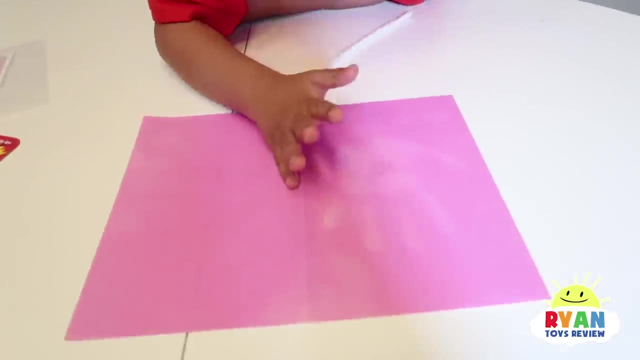 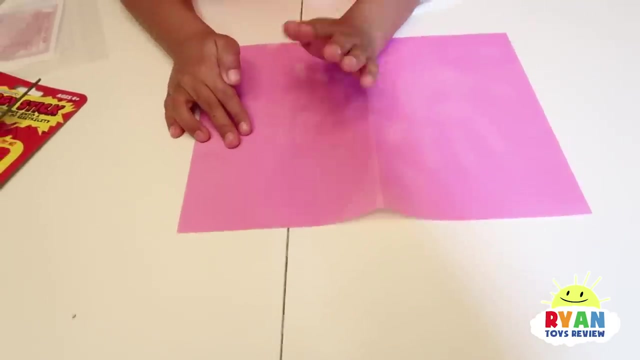 what happens There you go Now. hold it for a few seconds, Now let it go. What happened? My hand, Your hand, yeah, So this is like a special paper. It changes color when the temperature change. So that's pretty cool. Wow, All right, Mommy's. 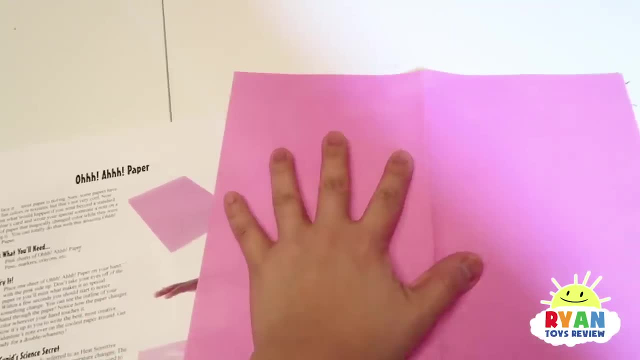 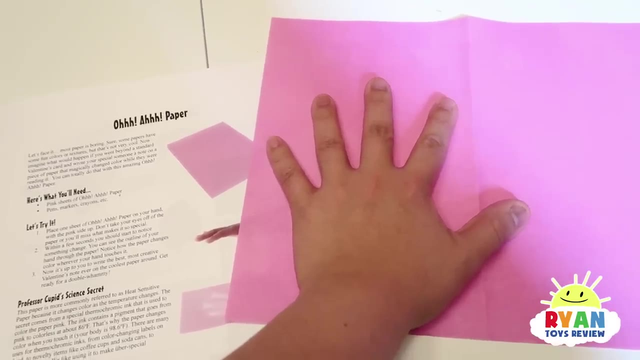 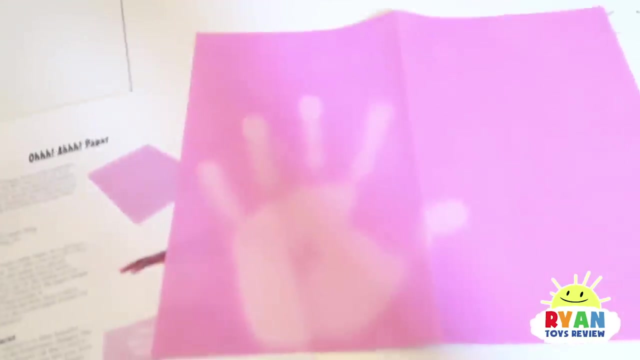 going to try. Let's see you guys, Look what happens. Bah, This ink contains a pigment that goes from pink to colorless at 98 degrees. What? Which is lower than your body temperature? Because your body temperature is 98.6.. So, wow, look at that. Next experiment, the love. 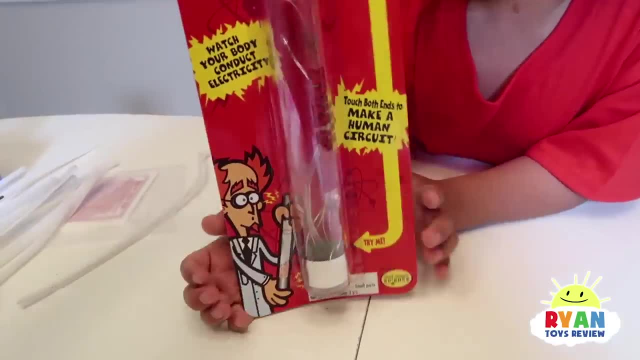 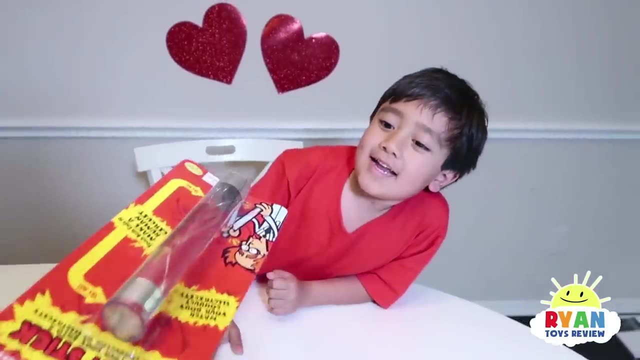 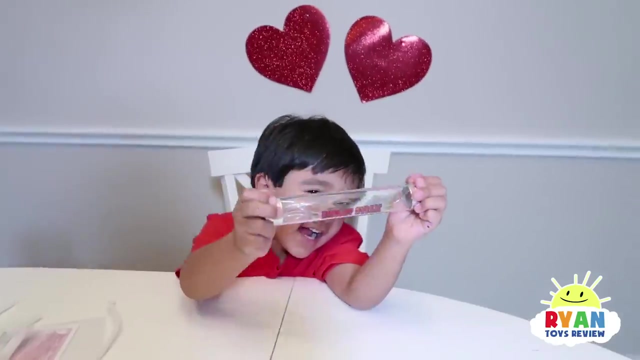 connection. So this is an energystick. It says: watch your body conduct electricity. So it doesn't work until we complete the circuit between Ryan and Mommy. Are you ready? Yeah, Okay. so Ryan holds one hand. it doesn't work, He has to complete the circuit with the other. 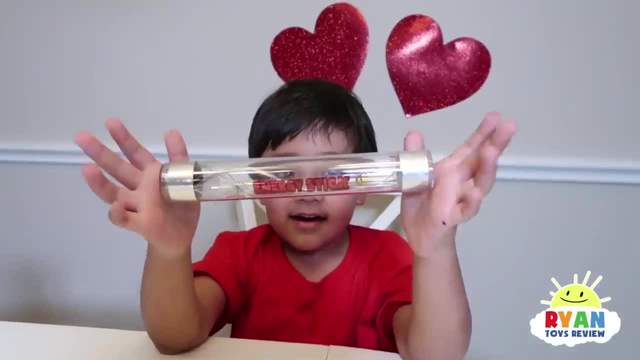 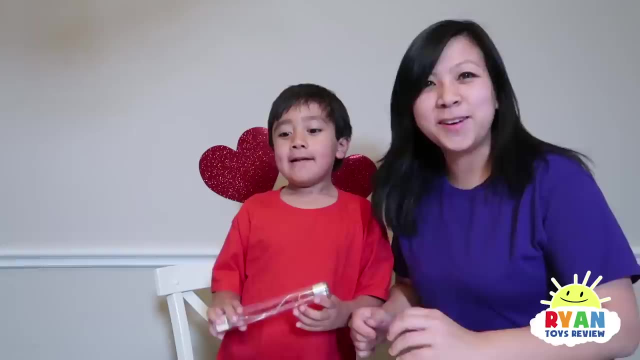 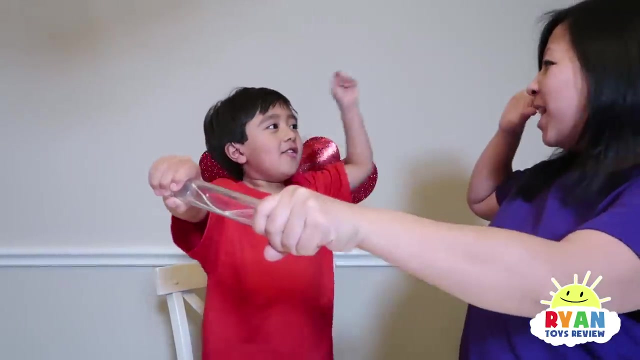 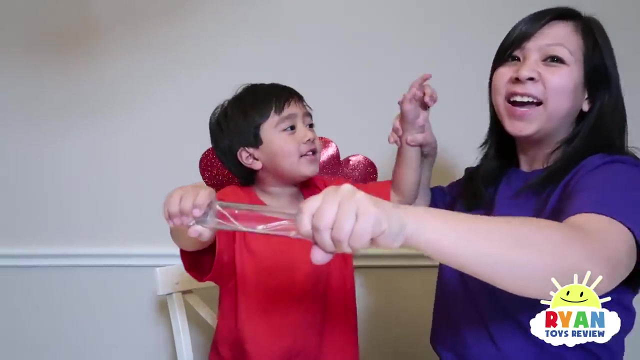 hand. Wow, Let's go push. Okay, let's go push. well, now mommy's gonna join, okay, so mommy and Ryan together doesn't work. you know how to make it work? well, how about your teeth? I don't think it works. I don't think so. 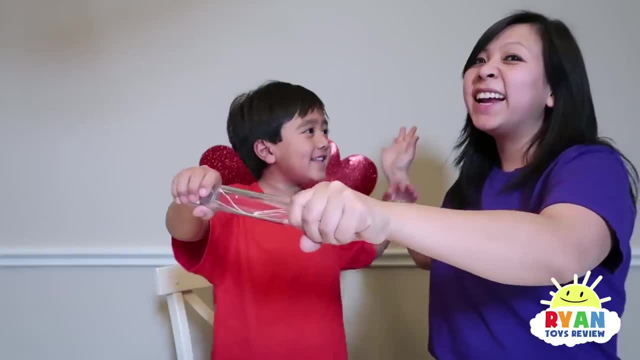 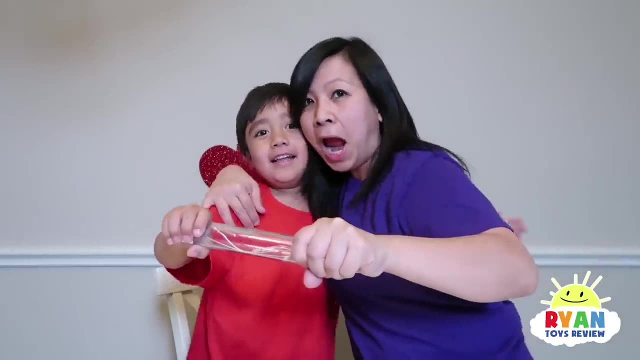 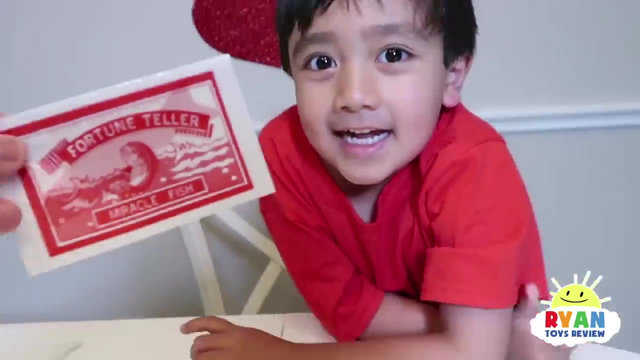 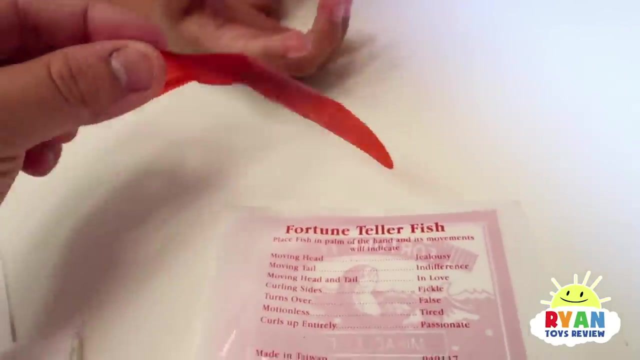 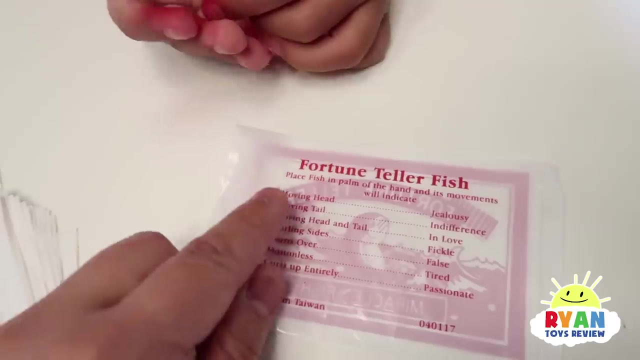 all right, once we let go and stop, once we hug each other. next we have the fortune teller fish. Wow, inside the fortune fish there's a fish. you see the fish? okay, so it says: if the head move, it means you're jealous and the tail move it means you're indifferent. and moving head. 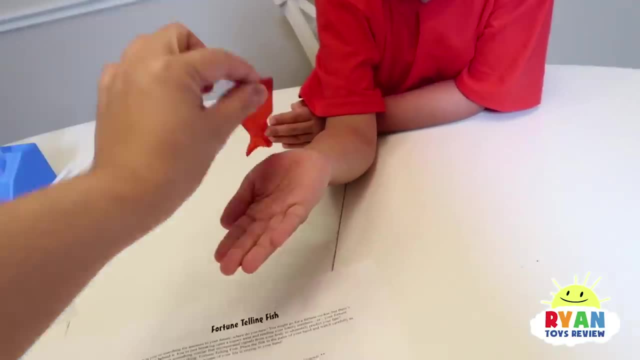 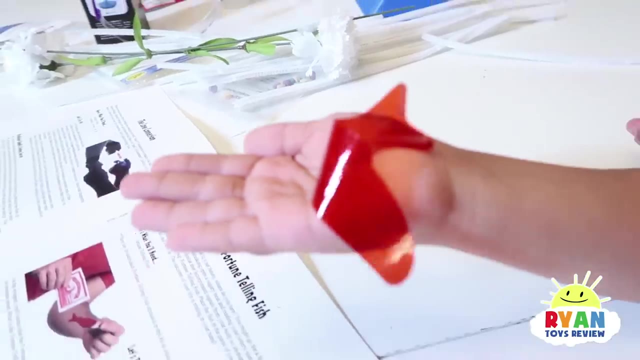 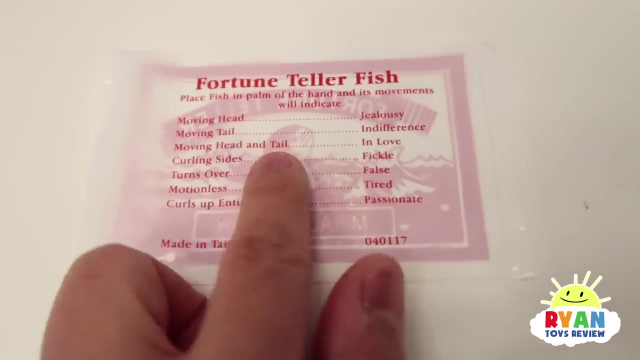 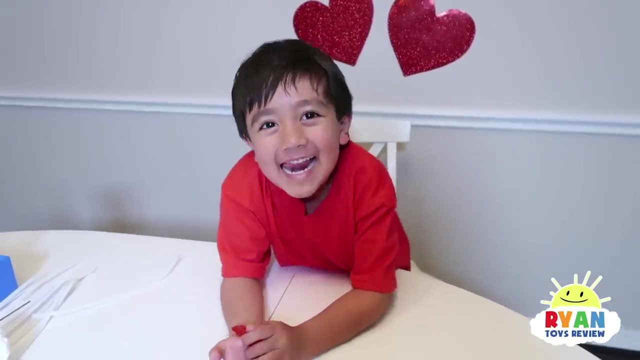 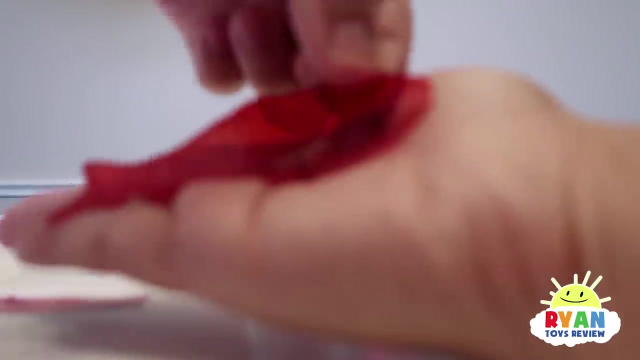 and tail. it means you're in love. let's see what happened to the fish. you have to wait. wow, yours curl. you see. no, your head move and your tail move. that means you're in love. Oh, Brian's in love. in love with the fish. mommy and daddy and Emma and Kate. is that why mommy's turn? let's see happen. 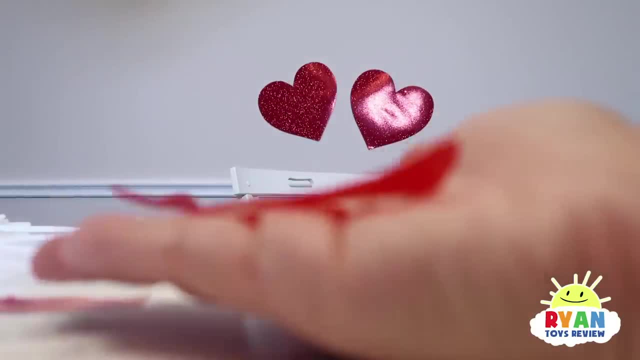 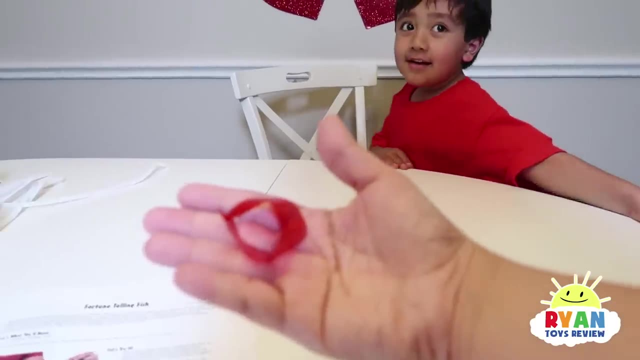 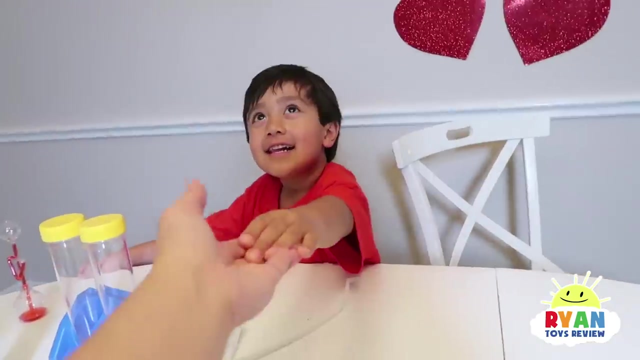 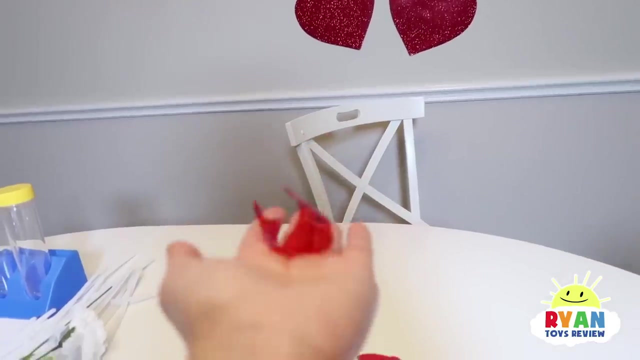 to mommy's fish. see anything, anything. oh, it curls both the tail and the head. that means mommy's in love with my family. how does it work? this curls because it touch moisture and your hand has moisture in it because your hand sweats, so my hands are sweaty. that's what it means, sweaty. 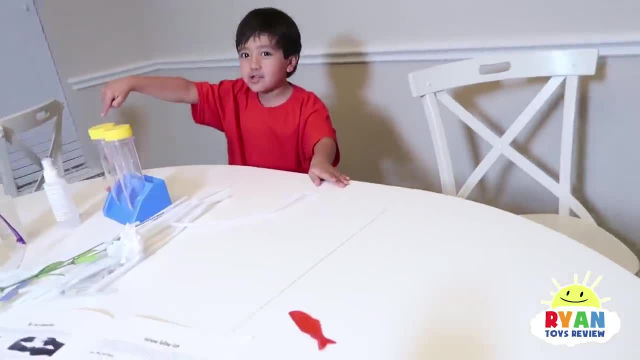 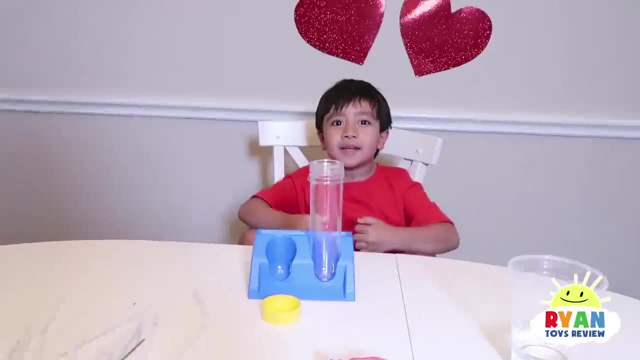 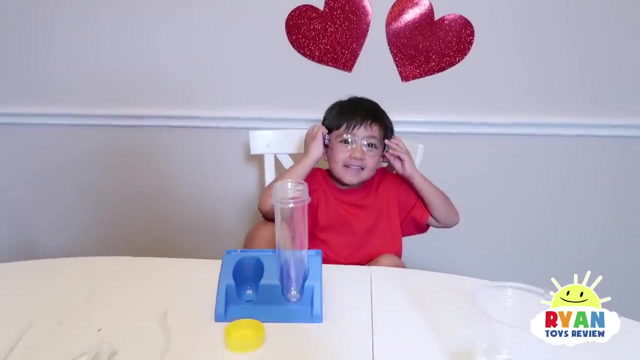 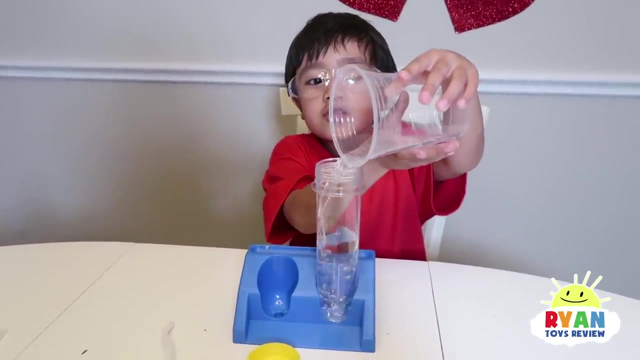 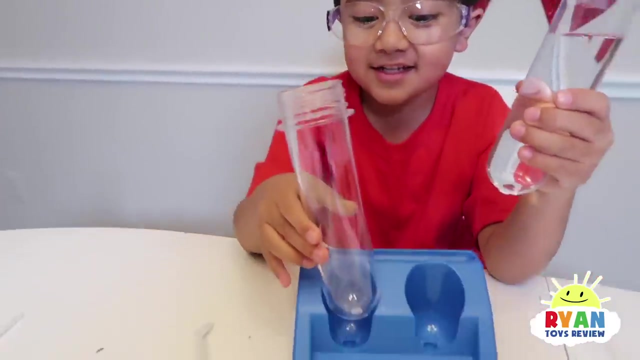 hands. yeah, so, mommy, have sweaty hands. that's what it means, sweaty hands. we gonna make a love potion. yeah, safety goggles this time. first, I'll put regular water to the test tube. next, I'm gonna pour the regular water into this empty test tube. yo guys, we'll. 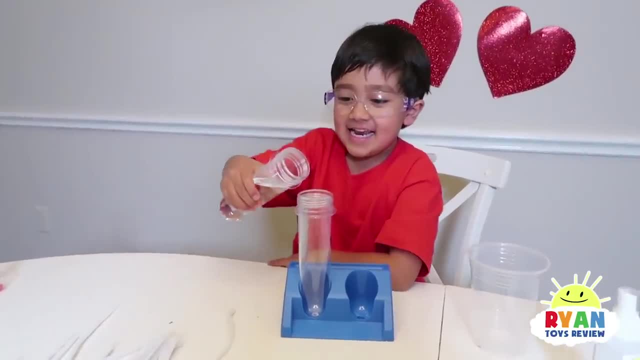 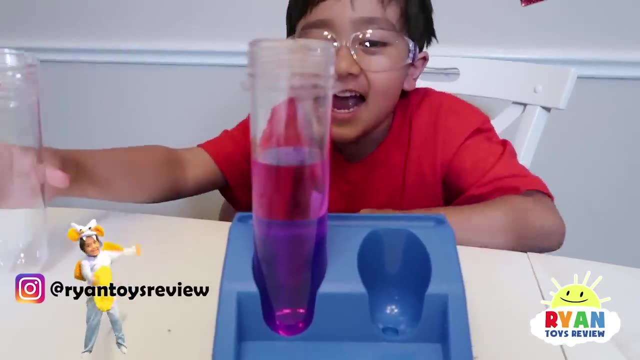 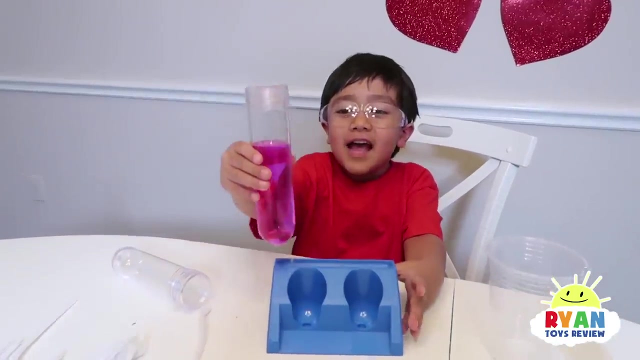 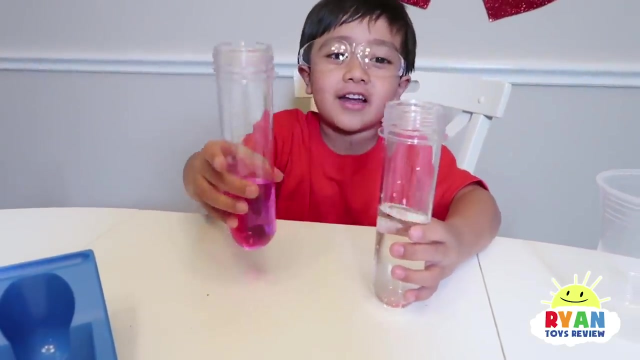 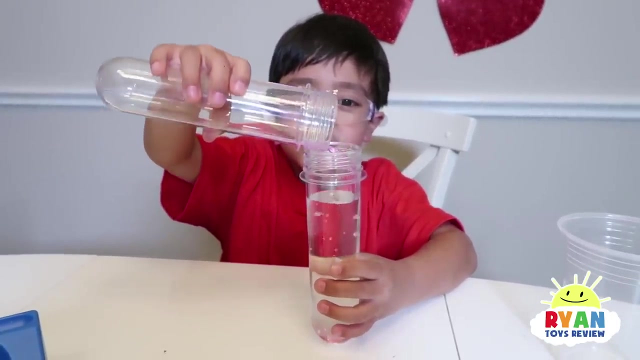 see what will happen. Ryan making a love potion. let's see. Wow, do you see what happened? yeah, it becomes pink. yeah, so it was clear water. now it's pink. this is my magical potion. we're gonna pour the pink magical potion into the vinegar. Let's see what happens. this is a type of acid vinegar and it will. 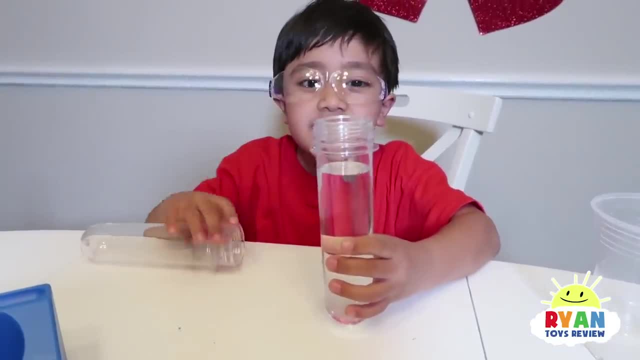 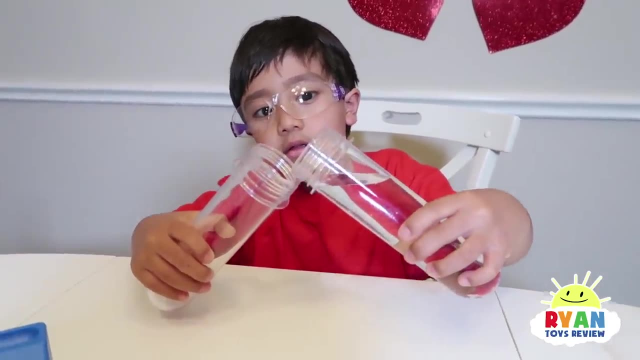 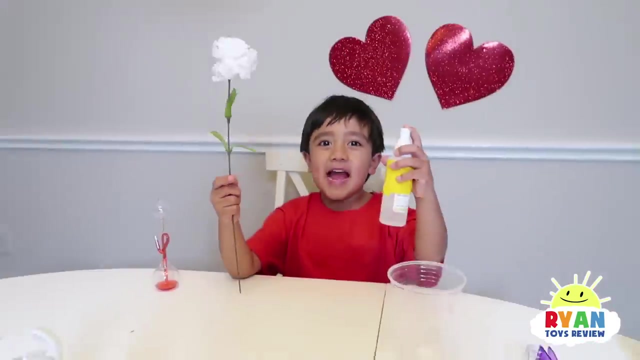 be clear. Wow, isn't that cool. so what happened? it will stay clear. so vinegar was an acid and this was actually a base, so they neutralizes each other. so that's why it turned back clear. if you know how he did it, leave it in the comments below, because magical potion this. 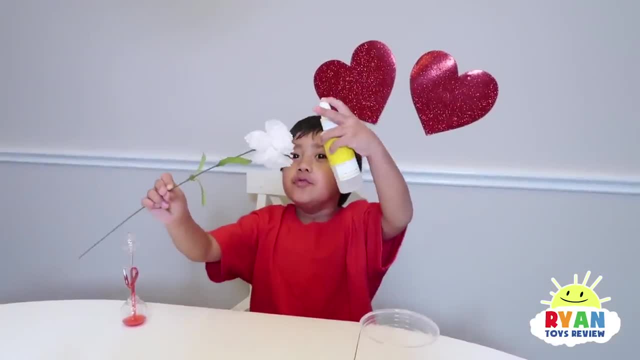 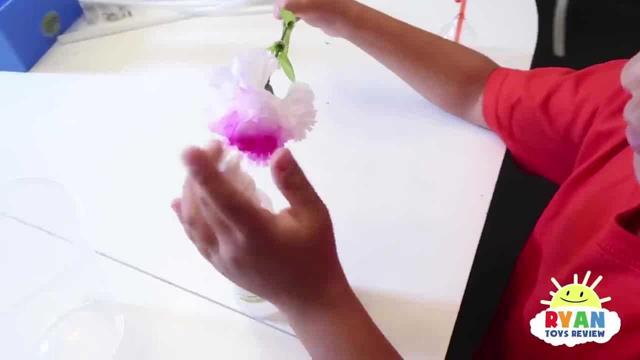 flower was amazing. guys, you guys are awesome, you guys are awesome, thank youle, and we'll. The flower will be turned into not white anymore, it'll be turned into pink. I'm just gonna spray this. Wait again, Oh, Wow. 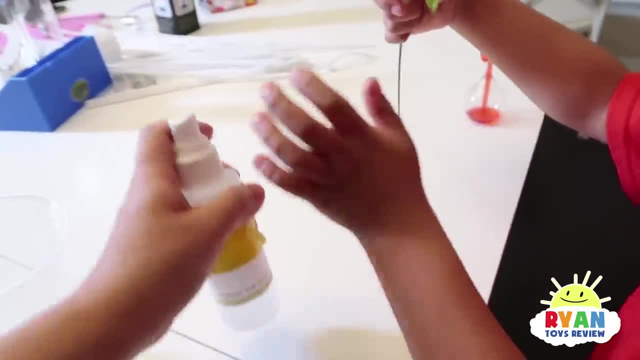 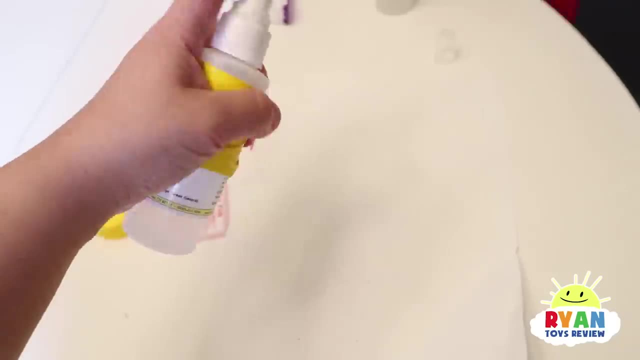 Oh, oh, oh oh. That's cool because this is actually clear. if you guys can see, Whoa, it turned super pink. see, Oh, it's flat. Yeah, so if I spray it on regular paper, it doesn't turn pink. 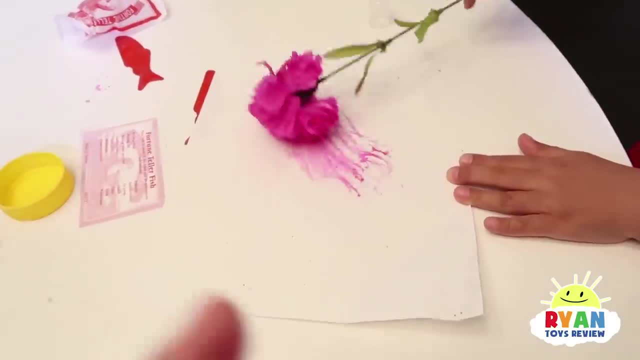 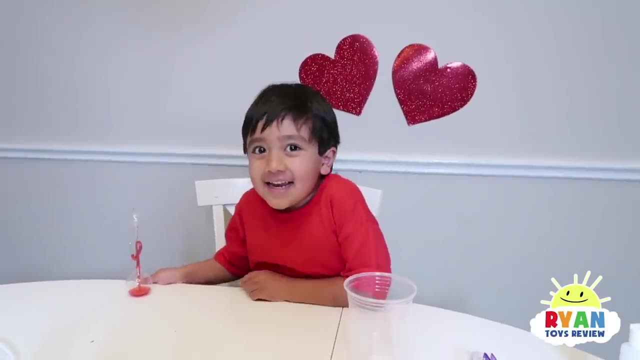 See, it stays white. If you put this on the regular paper, it turns white. Yeah, Whoa, Valentine magic. Yeah, You guys wanna know how we did it. Yeah, We actually sprayed this with phenolphthalein. 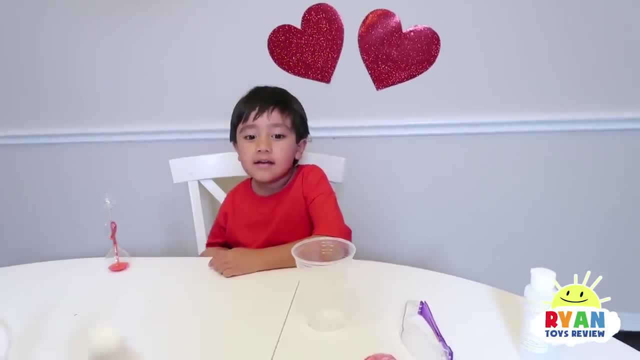 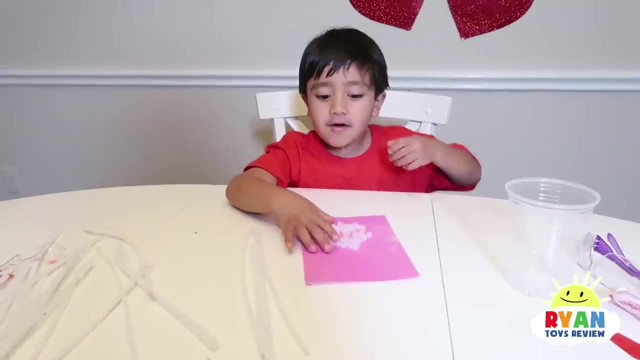 which is it will turn pink if it's a base. And what do we use as a magical potion? It's actually ammonia, which is a base Base, So it will turn pink, Pink. So I have these magic beads. 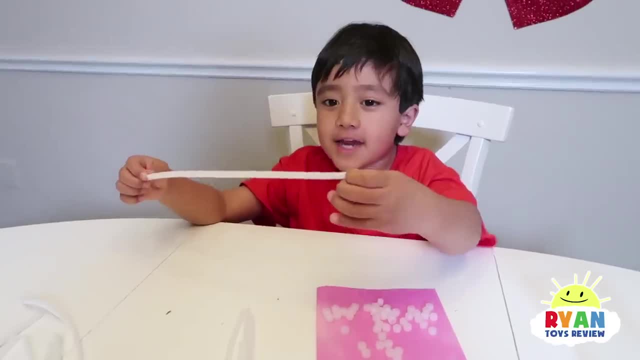 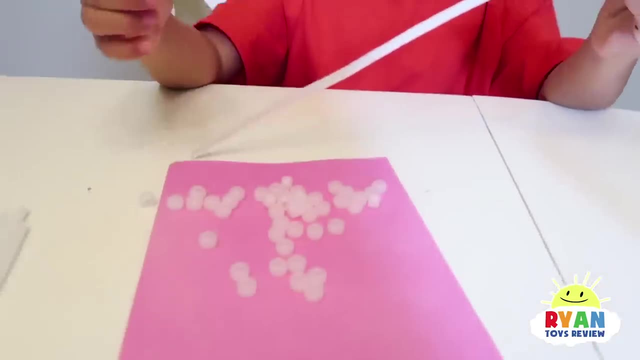 where, if you put these on this bracelet, make a bracelet and put it in the sun, it will turn pink. Ryan's gonna build his bracelet Right now. it's white. All this stuff are white, so it's kinda like it's blending in. 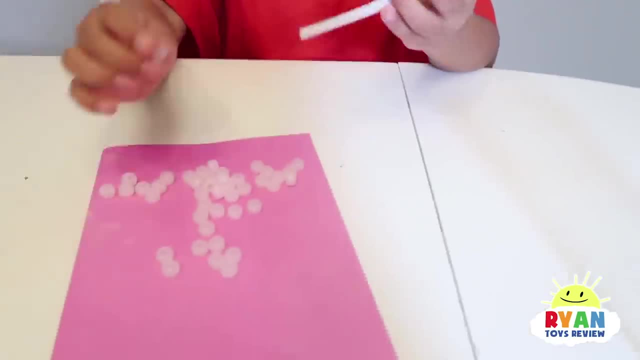 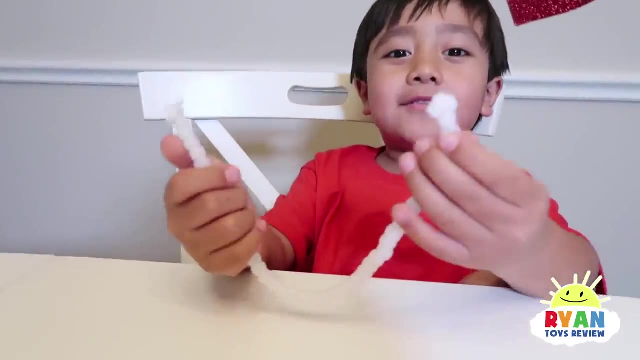 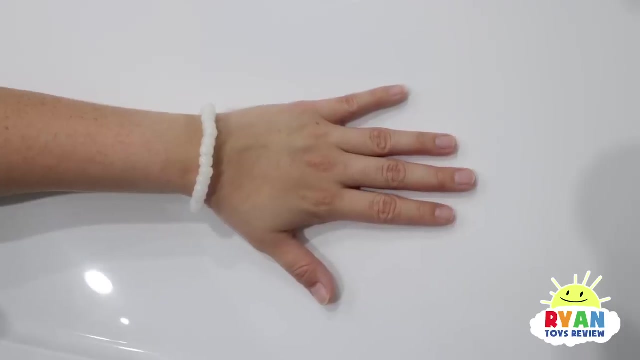 Yeah, Might take one hour. My bead is complete. Now let's take it out to the sun. There it is, right now it's white bead that Ryan just made. Oh wow, look at the bracelet. It's turning color under the sun. 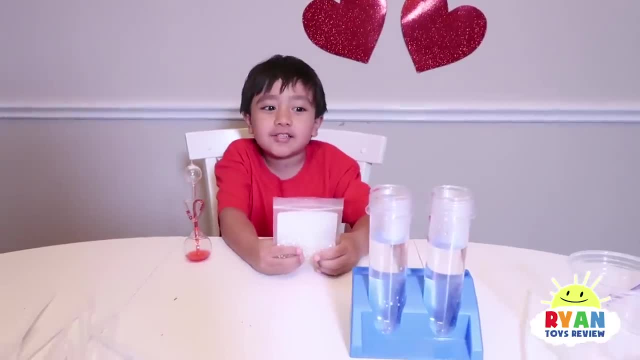 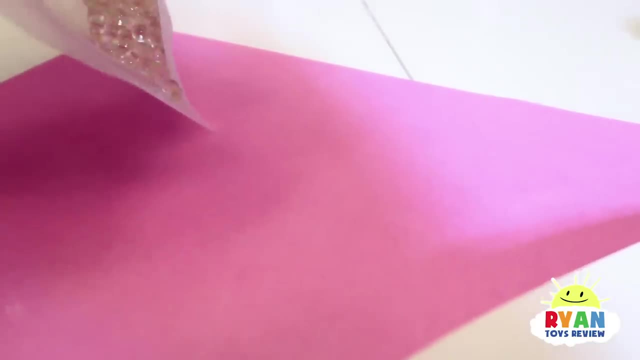 That's awesome. Now we're gonna grow some jelly marbles. These jelly marbles are really really super tiny. They are like Orbeez. Whoa see, they're super, super tiny And we're gonna drop it into the test tube. 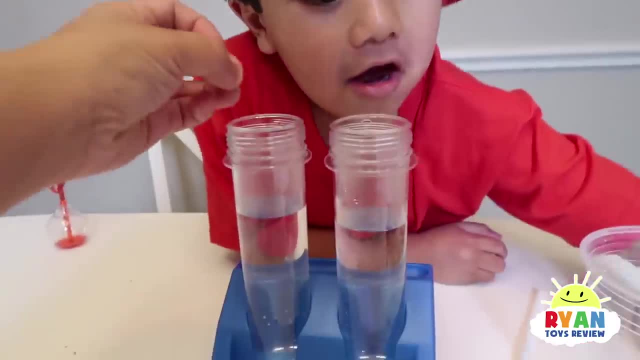 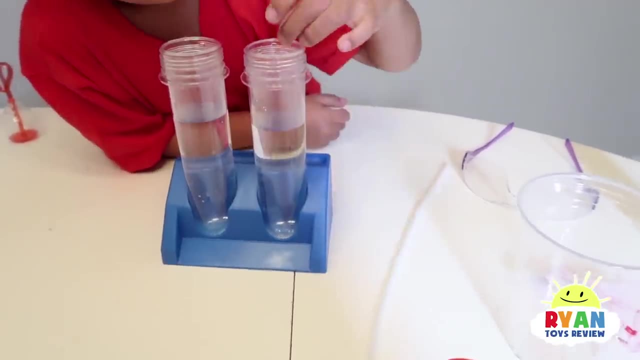 and we're gonna wait eight hours- Eight, Yeah, and then it's gonna grow super huge. Look how small they are now. Drop them in the test tube. I think we need a lot. Yeah, Okay, Ryan, which color changing do you want? 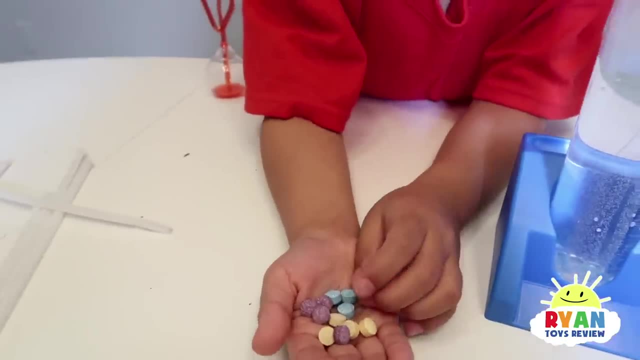 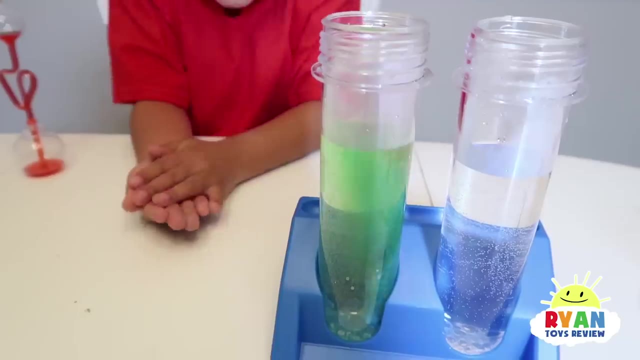 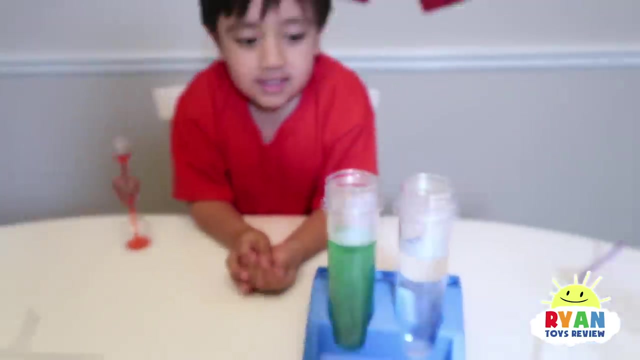 Which tablet you want to change colors: Blue, Blue. Okay, Can we do two? Yeah, sure, Blue and yellow will make green. Wow, We're gonna change that one to green and we're gonna leave that one to white to compare, okay. 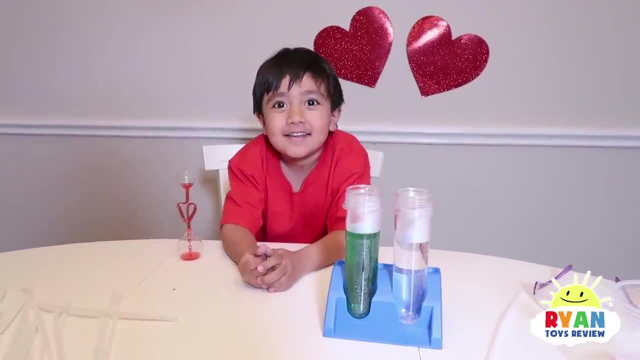 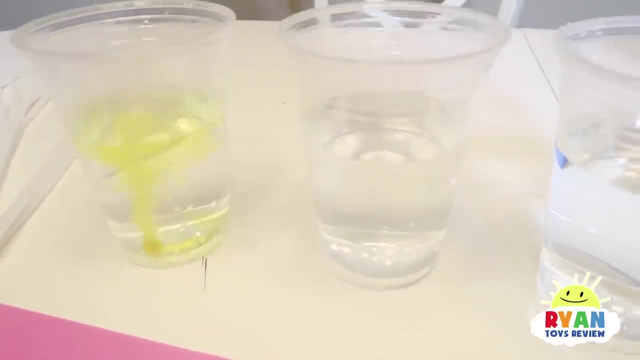 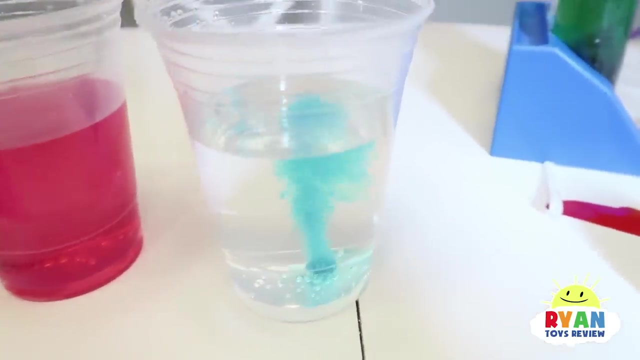 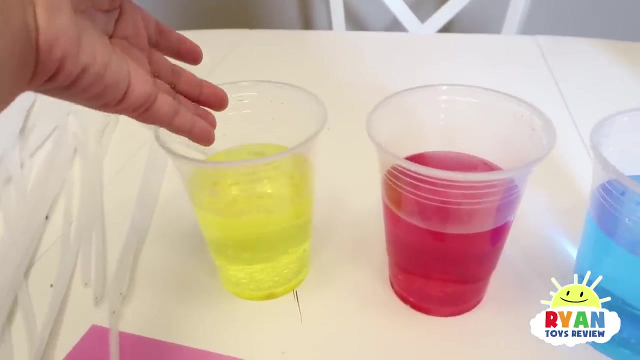 See you in eight hours. See you in eight hours, Well, tomorrow morning, right? Yeah, We're also going to use the different color tablets so we can make all different colors. There's yellow, pink And there's blue. Wow, I'm gonna drop some jelly into the yellow. 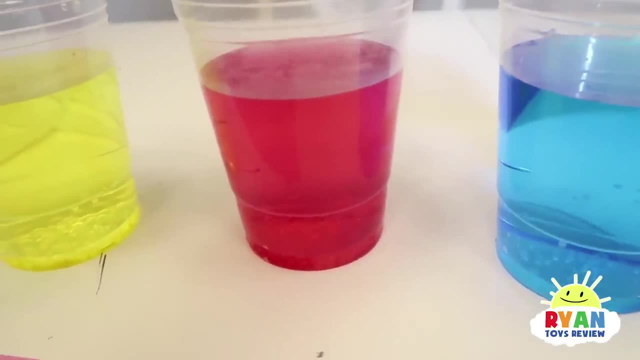 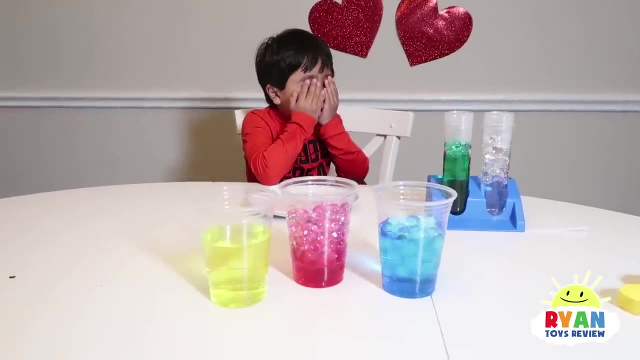 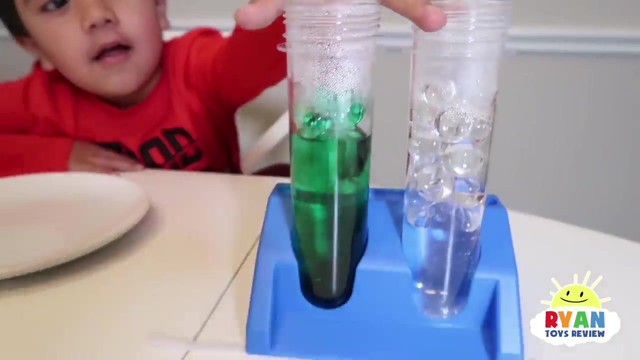 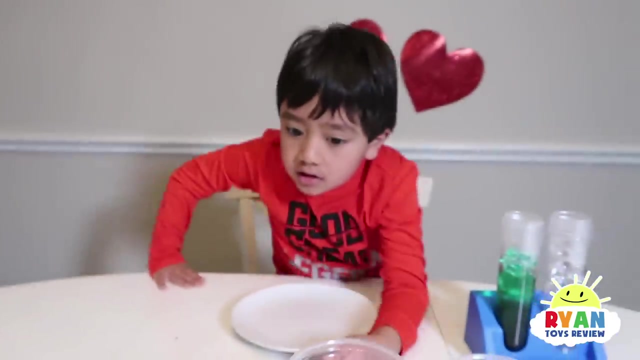 Drop some in the pink, Drop some in the blue. We'll wait for eight hours, So it's the next morning. You want to look now? They look like ice cubes. Look how big they gone. They're so huge What. they definitely look like Orbeez and I feel like they feel like Orbeez. It's hard to see yellow.